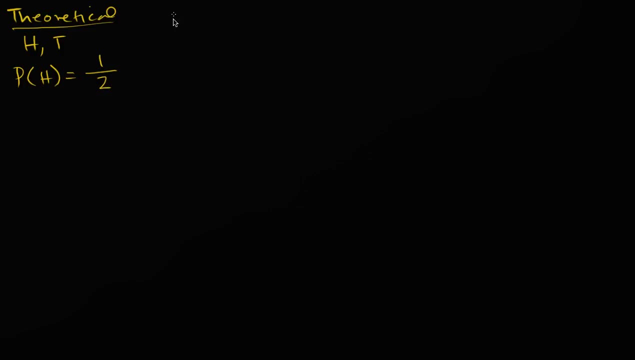 We could also do that with rolling a die. A fair, six-sided die is going to have six possible outcomes: One, two, three, four, five and six. And if you said, what is the probability of rolling or getting a result that is greater than or equal to three? 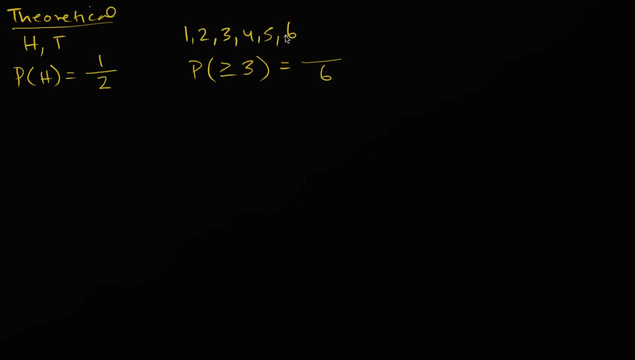 Well, we have six equally likely possibilities. You see them there And, in theory, if they're all equally likely, four of these possibilities meet our constraint of being greater than or equal to three. So we have four out of the six equal of these possibilities. 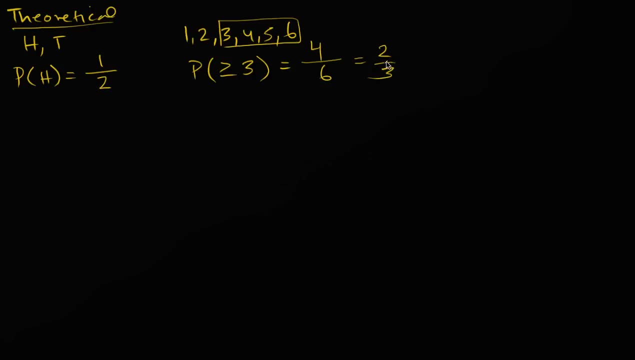 meet our constraints. So we have a two-thirds- four-sixths is the same thing as two-thirds- probability of it happening. Now, these are for simple things like die or flipping a coin, And if you have fancy computers or spreadsheets, you could even say: hey, I'm going to flip a coin. 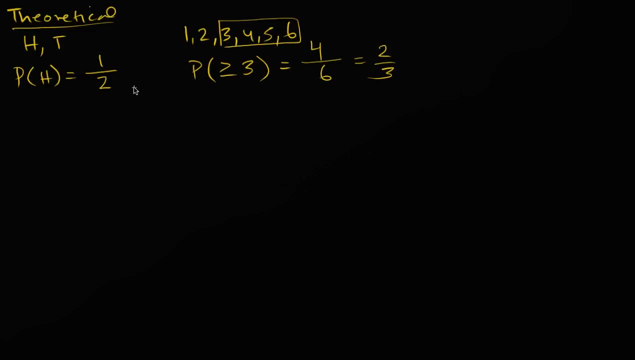 a bunch of times and do all the combinatorics and all that, But there are things that are even beyond what a computer can find: the exact theoretical probability. Let's say you're playing a game, say football, American football, and you wanted 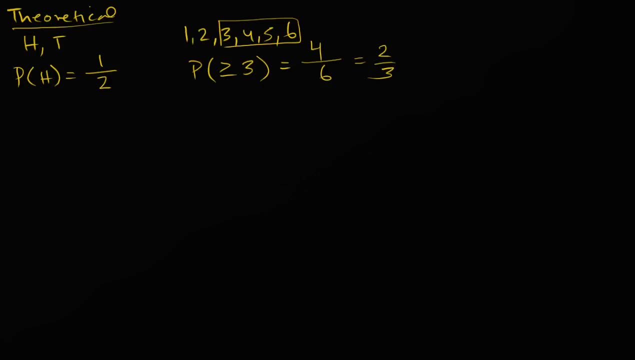 to figure out the probability of scoring a certain number of points. Well, that isn't very simple because that's going to involve what human beings are doing. Minds are very unpredictable How people would respond to things. the weather might get involved, someone might fall sick. 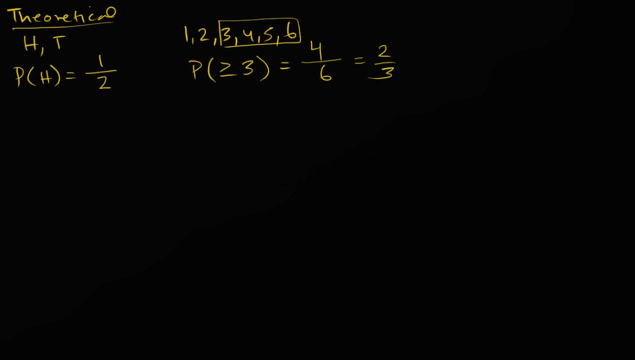 the ball might be wet, or just how the ball might interact with some players, the jersey, Who knows what actually might happen, What might actually result in the score being one point this way or seven points this way, or seven points that way. 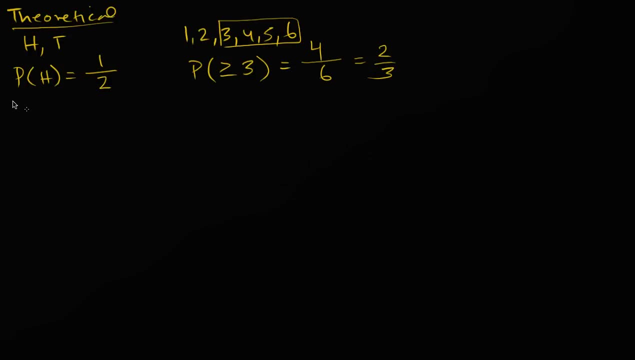 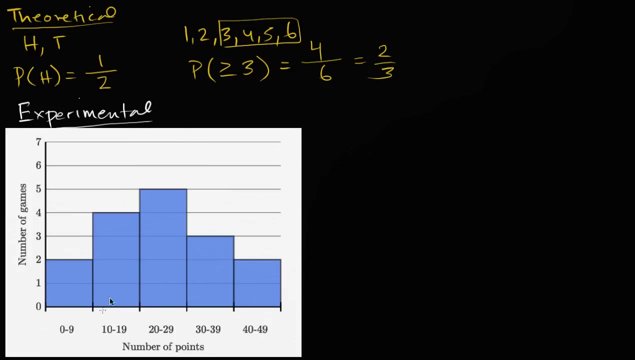 And so for situations like that, it makes more sense to think more in terms of experimental probability, And experimental probability: we're really just trying to get an estimate of something happening based on data and experience that we've had in the past. So, for example, let's say that you had 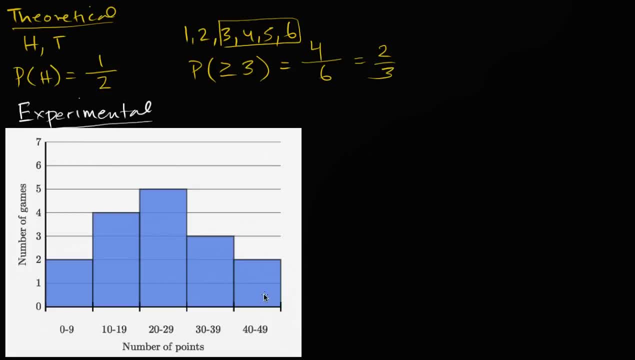 this is data from your football team and it's a game, It's a couple of games or many games into the season And you've been tabulating the number of points. You have a histogram of the number of games that scored between 0 and 9 points. 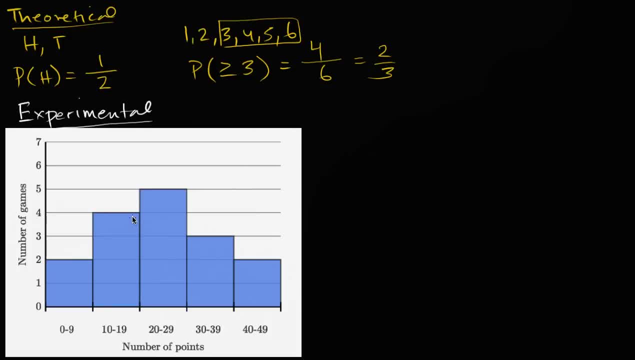 You had two games that scored between 0 and 9 points, Four games that scored between 10 and 19 points, or from 10 to 19 points. You have five games that went from 20 to 29 points. You had three games that went from 30 to 39 points. 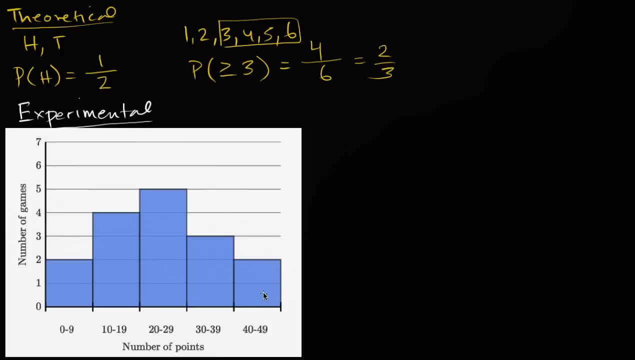 And then you had two games that go from 40 to 49 points. And let's say, for your next game you've already had two. Let's see how many games you've had so far. this is two. let me write it down. 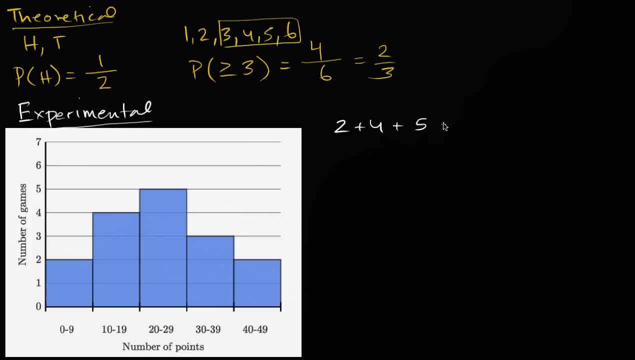 The game so far is two plus four plus five plus three plus two. so this is what six plus this is. six plus five is 11, 11 plus five is 16.. So you've had 16 games so far this season. 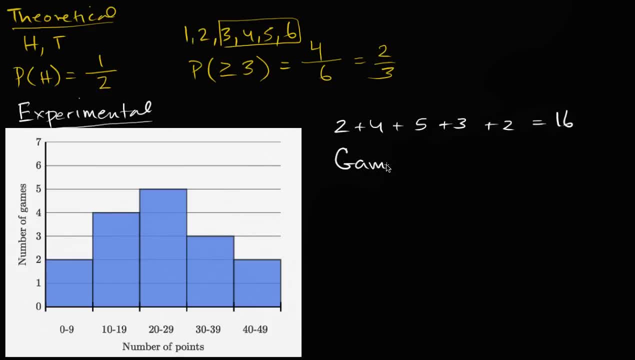 And you're curious for your 17th game, so let me write this game 17,. you want to figure out what is the probability of scoring, scoring, scoring, let's say score, let's say your score, let's say your points. 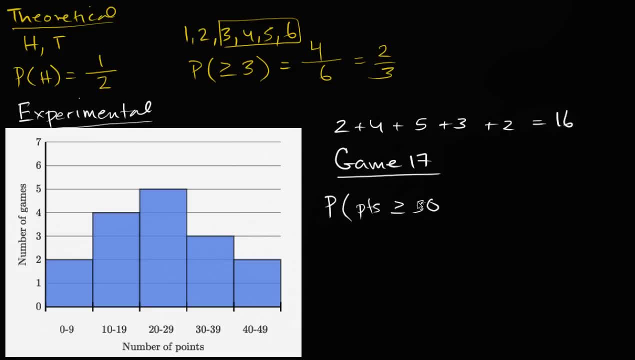 your points are greater than or equal to 30.. Your points are greater than or equal to 30 for game 17.. So, once again, this is very hard to find the exact theoretical probability. You don't know exactly, you can't predict the future. 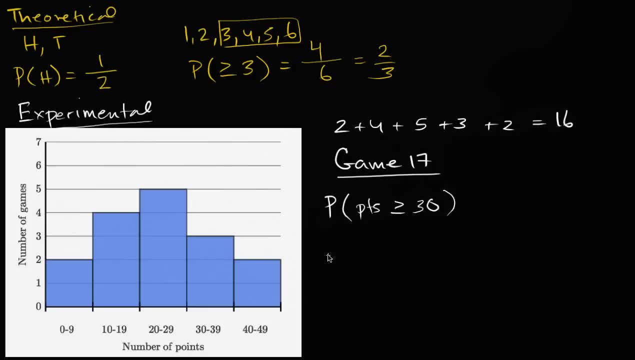 You don't know who's gonna show up sick, how humans are going to interact with each other. maybe someone screams something, something in the stand that just phases the quarterback in exactly the right or the wrong way. You don't know. this is an incredibly 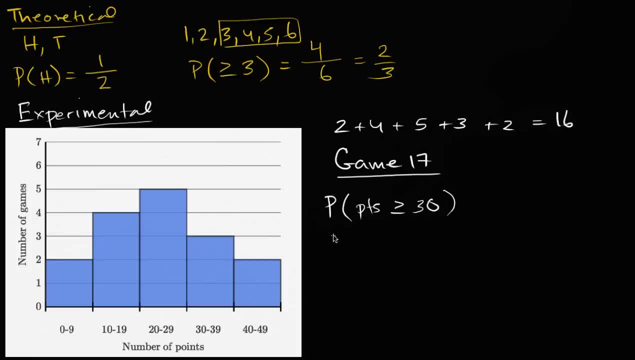 incredibly complex system, how what might happen over the course of an entire football game. But you can estimate what'll happen based on what you'll see in your past experience And it depends on the defense of the team you're facing. and all of that. 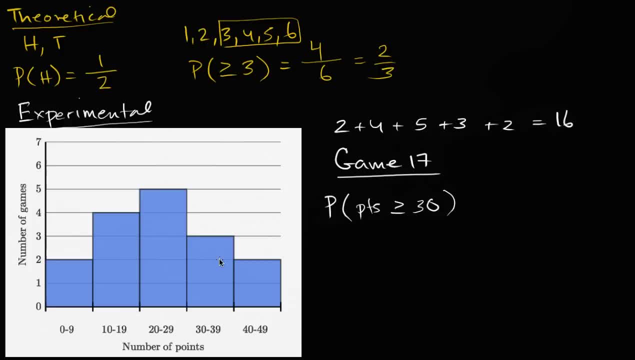 So it's not going to be, you know, it's not going to be super exact, but you can estimate based on experiments, based on what you've seen in the past Here the experimental probability and I would say the probability, the estimate. 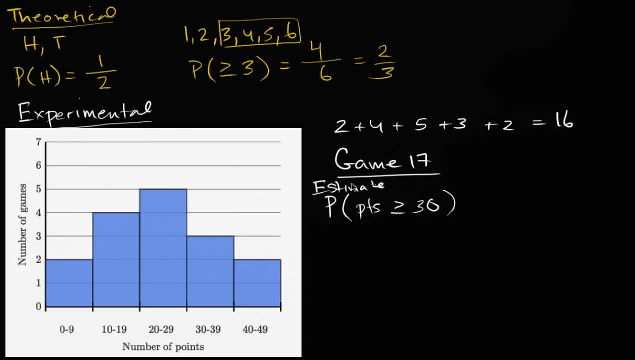 because I would you know you shouldn't walk away saying this. okay, we absolutely know for sure that if we conducted this next game experiment n times, it's definitely going to turn out the same, Because this might be the toughest defense that you play all year. this might be the easiest defense. 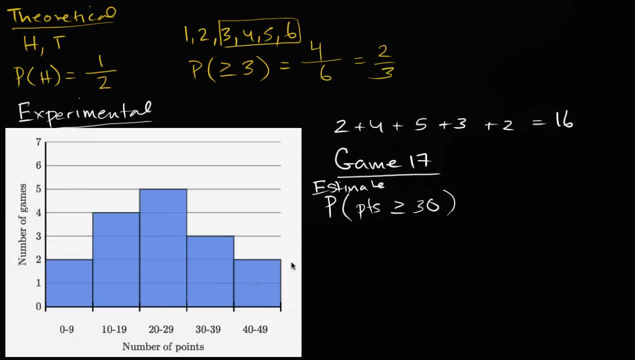 that you play all year. But if you look at what's happened in the past, out of the 16 games so far, there have been three games. these three plus these two games where you scored more than, greater than or equal to. 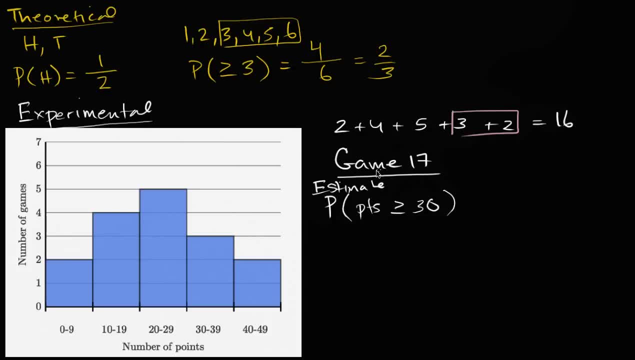 30 points, So five out of the 16 situations you've scored more than that. So an estimate of your probability and you could view this as maybe your experimental probability of scoring more than 30 points based on past experience. based on past experience: 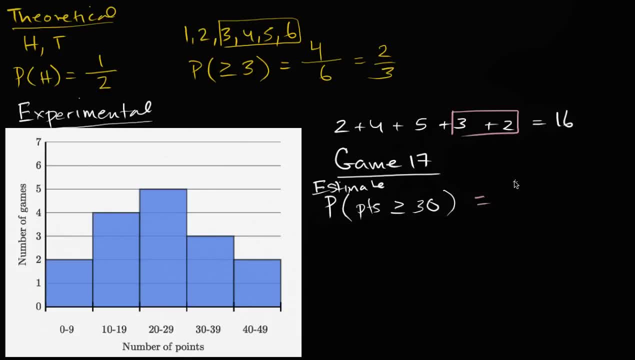 is five, five out of the 16 games. you've done this in the past, So you'd say it's five, sixteenths. Now I want to really have you take this with a grain of salt. You should not, you know, then go. 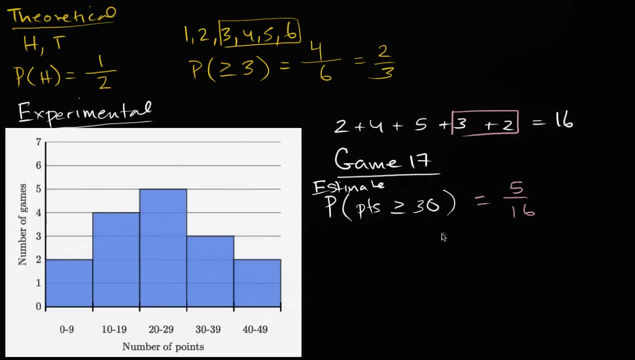 say: okay, I know for sure there's a five sixteenths probability of us winning this game, Because you only have some data points. every team you play is going to be different. it's going to be different weather conditions, people are going to be in different moods. 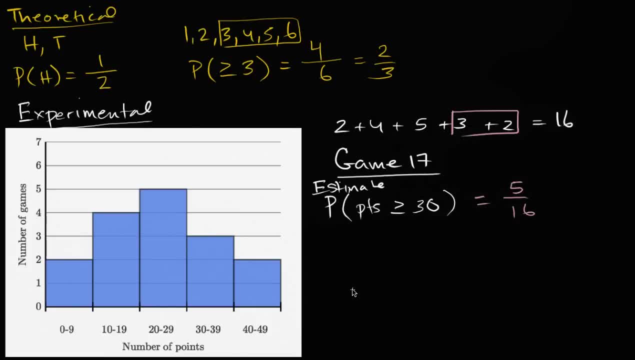 et cetera, et cetera. This is really just an estimate. I actually, I feel even a little bit of reservation is even calling it a probability. I would just say that this has been true of five out of 16 games in the past. 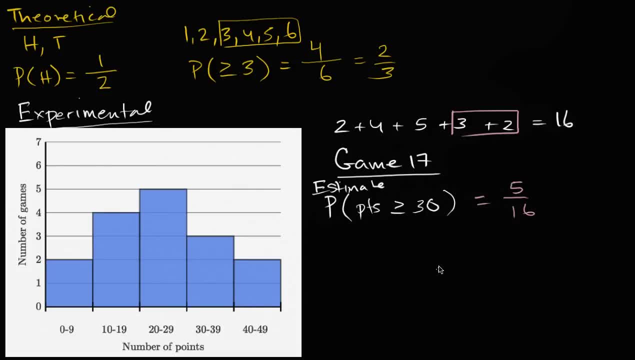 so it's an indicator of what might be what you know. you might say, oh okay, based on experience, it's more likely than not that we don't score more than 30 points. But it's really just based on experiential data.